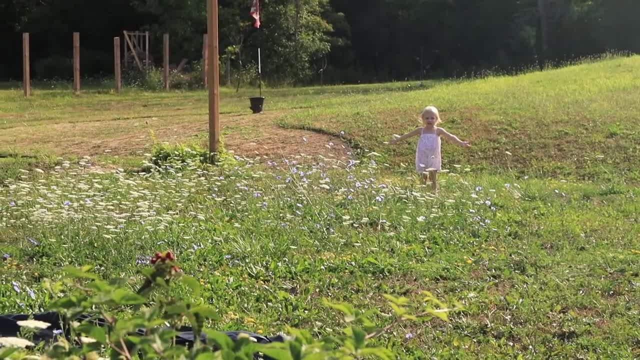 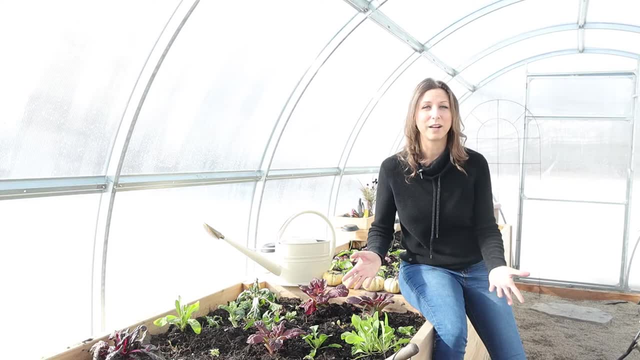 But, that being said, if you have a garden and you have kids and you've seen success with some of the things that you like to do with them, throw a comment down below and I think maybe we can get a pretty good list going between what I have in this video and your suggestions as well. 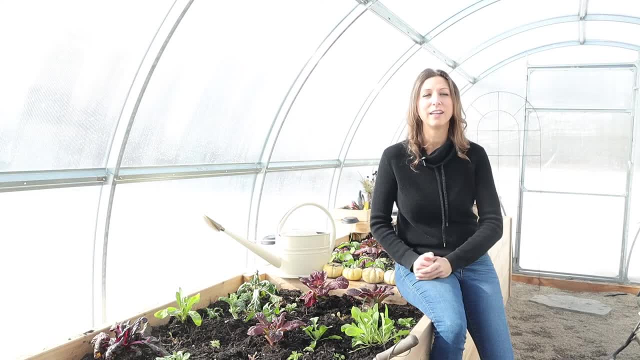 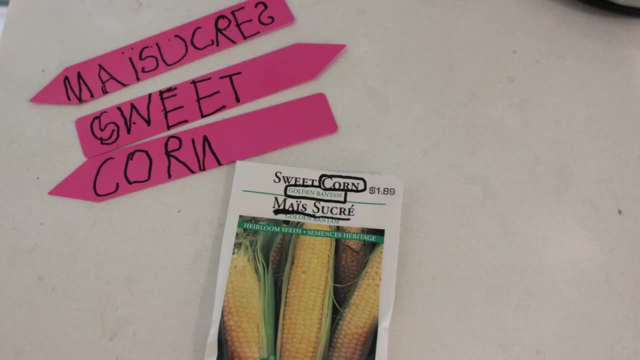 The first thing I like to do with my older daughter in particular is help me write out the plants on the plant labels. So my older daughter, she's in kindergarten now she's five and she's learning how to read and write and I thought when I was starting my seeds, I showed her the seed packet. 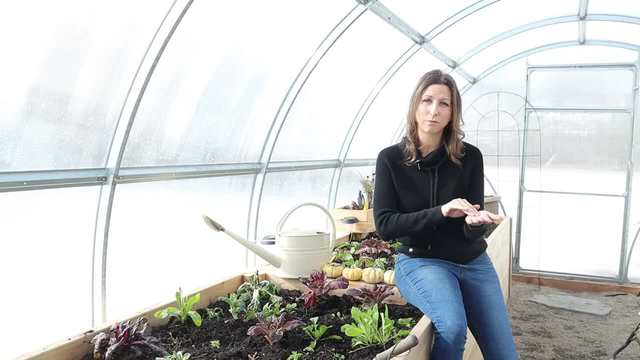 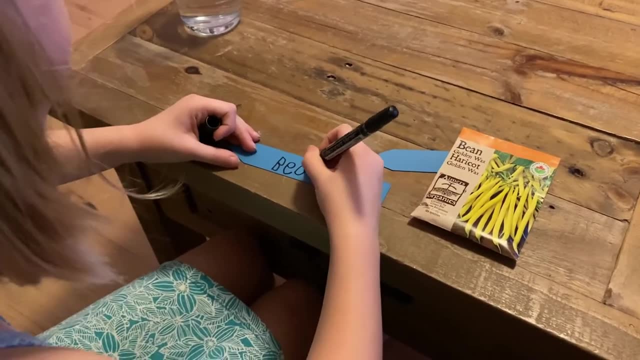 and I said, you know, I underlined the word that we were writing so and you know there's lots of words on a seed packet, so I underlined the word in particular that I wanted her to write and she copied it out onto the seed packet and then, you know, it usually took up the whole plant list, but I 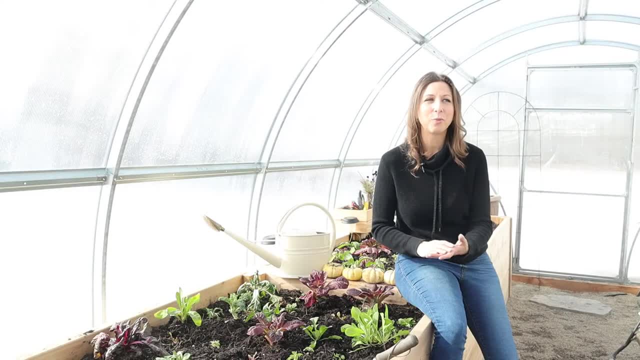 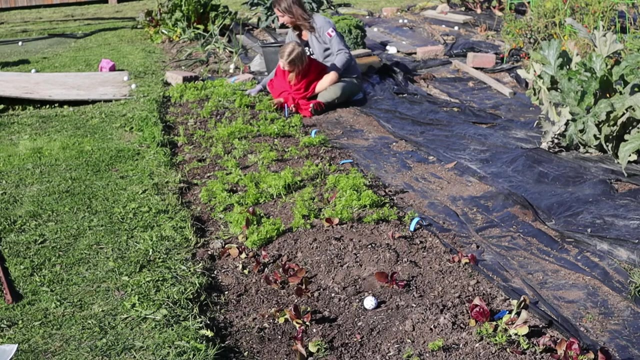 thought that was pretty cool. Another thing that, surprisingly, my kids love is weeding. It's a weird thing for a kid to love, right Like. I don't remember loving weeding as a kid. My parents didn't have a like a vegetable garden necessarily. growing up. We had a bunch of fruit bushes, but 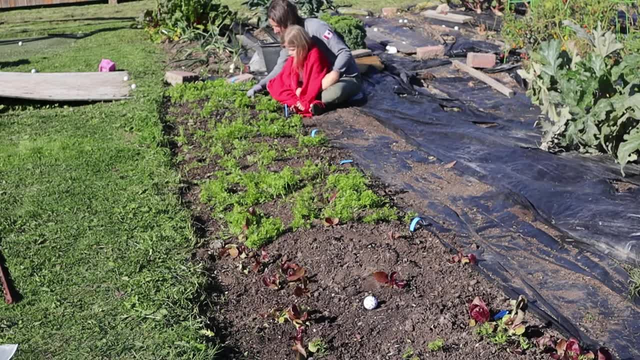 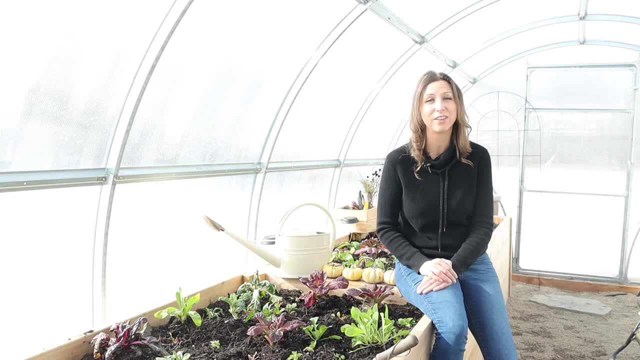 I didn't really ever have the task of weeding, so I can't really say whether or not I would have loved it or not, but I don't feel like I would have loved it. I don't feel like I would have loved it as a kid but surprisingly- and I've heard this from other parents as well- like they, they actually 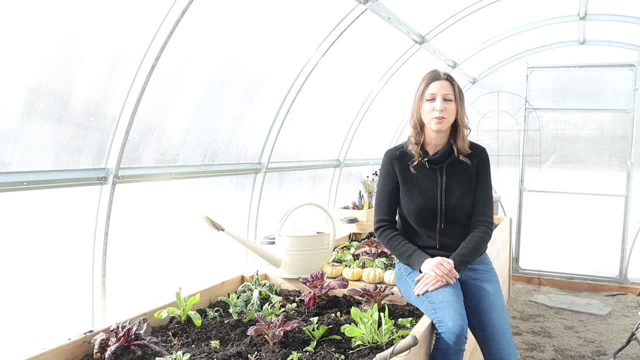 their kids like weeding, or they liked weeding as a kid. so I think that it's just a matter of kind, of how you phrase it and whether you do it with them. So I use a hoe, like, and I'll have a link to the kind I use. It's awesome. It makes weeding so easy. but I use this hoe and when I do weed with it. 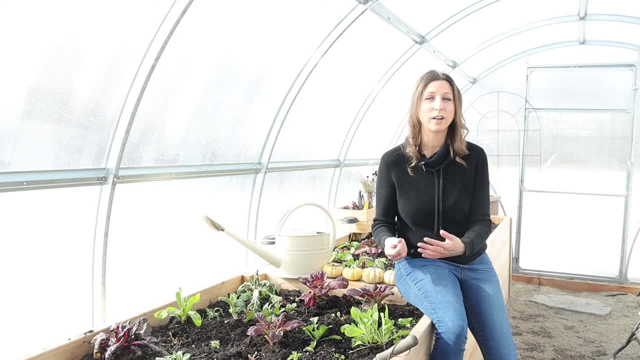 they always try to grab it from me. They always try to take it and want to take turns, which of course makes weeding go very slow, But it's you know. it's the kind of thing that you'd be surprised when you start doing something. 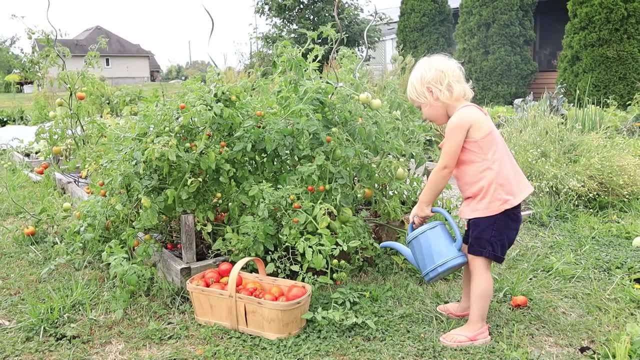 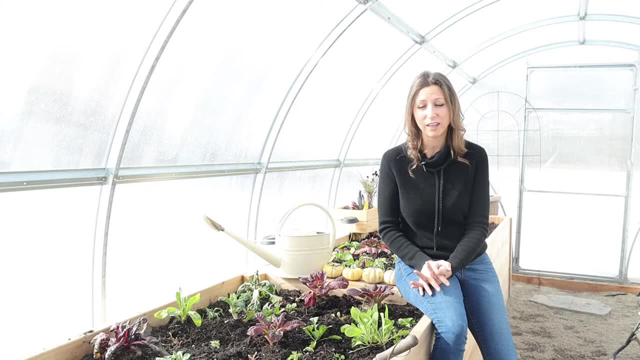 in the garden. Watering is another one. Weeding and watering are two kind of garden tasks that not everyone loves, but kids really do like those things. It's something that they can do. They can see the result of what they're doing. like if you're weeding, you can see the difference before. 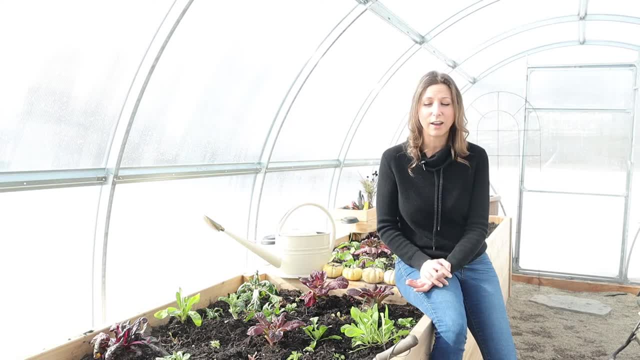 and after very fast, and the only thing I have to say, though, about both weeding and watering- if you want to get your kids involved in those, is to give them tools that work. Don't give them necessarily just like plastic or just like tools that might. 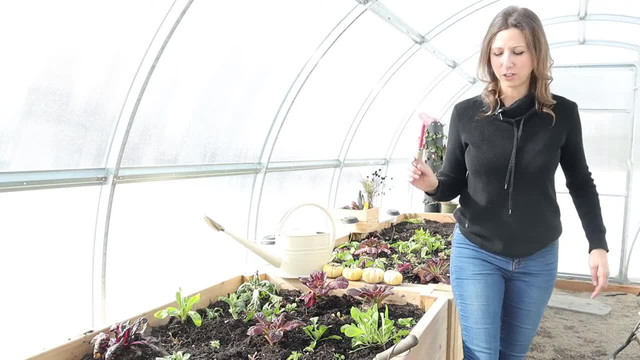 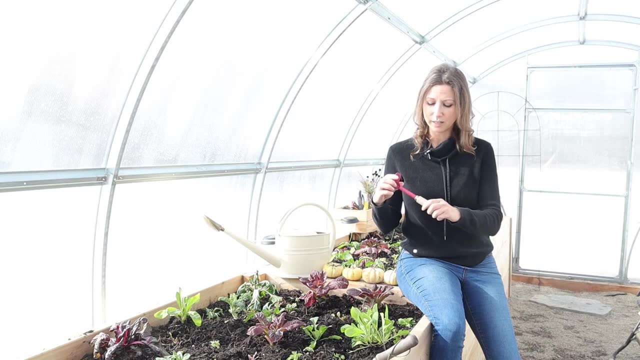 break. I have a like. I got my daughter these kind of little. this one's actually not too bad. This one is has a wooden handle and it's metal, but it will break if she tries to use. I don't use this very much in the garden, so she doesn't really use this. They use the exact same tools that I do. 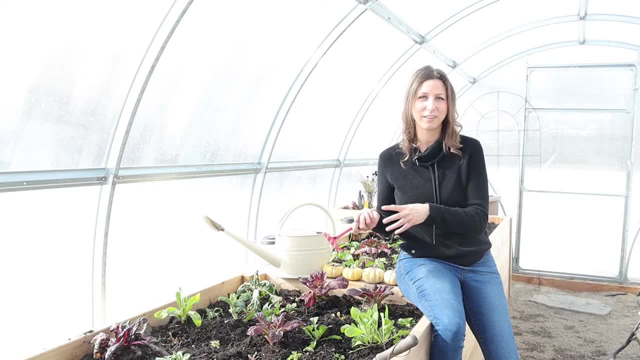 So if you're going to try to find a kid-sized version of something that you use, Try to make it look very similar. It can be different colors, but try to try to make it look the same, because if I'm using something with a flat edge, she doesn't want to use something that has a fork. 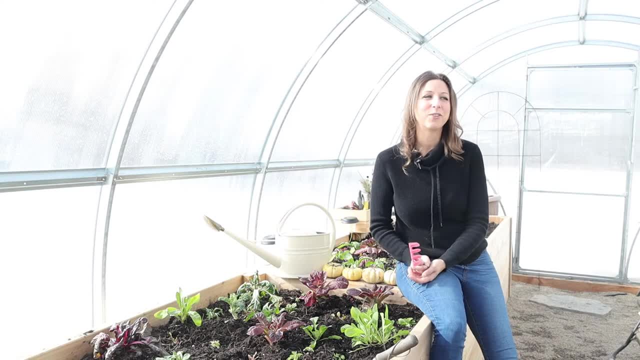 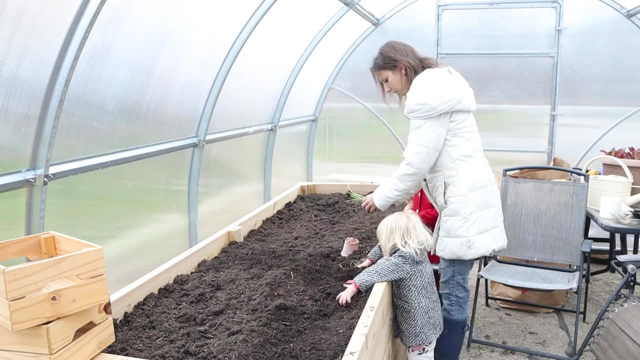 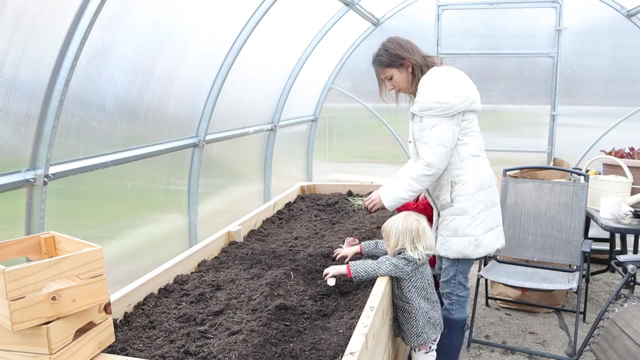 egg fork edge like this. They want it to be the same. So try to find something that is will do the same job as yours and that way you can both be using the tool at the same time. And this obviously is more applicable to like a little kid, where you would be doing it with them. An older kid can just 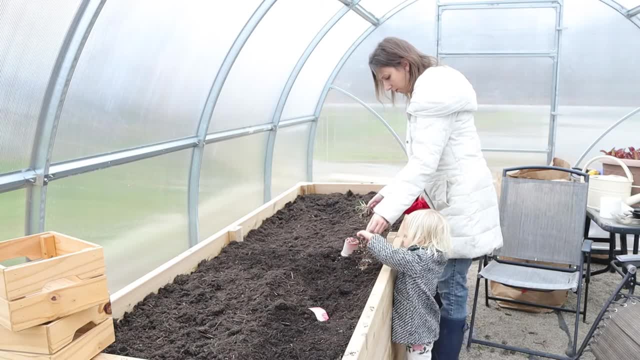 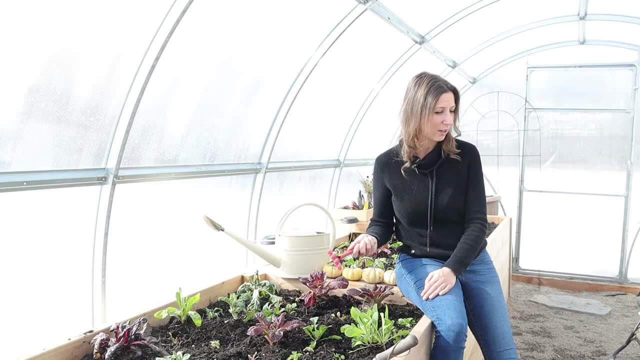 use your tool, of course, But if you're a little tiny kid, I would give them tools that are cute, that they love, that actually work. I had I don't remember I don't. I mean I would have thrown it out, but it was kind of like this. but as 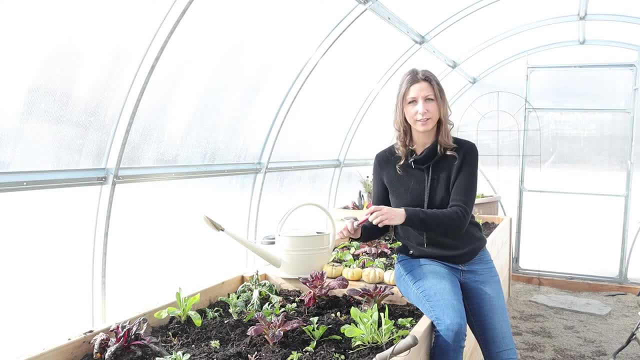 soon as my daughter stuck it into the soil and she tried to do what I was doing, it just snapped off because it was like a. it was just a toy. it wasn't actually a garden tool. and kids are strong- right, they're strong. they will actually go in and try to do what you're doing. So I mean, I've had adult 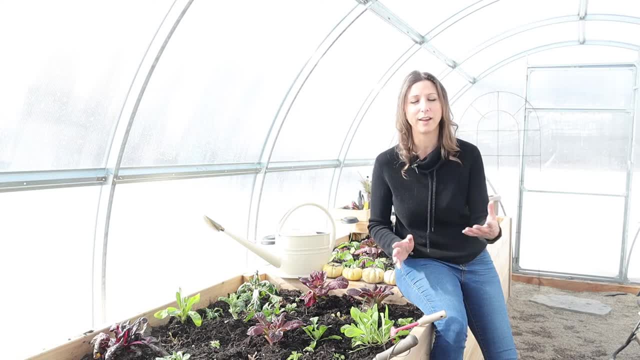 made tools break for me in the soil, which is why I tend to spend a little bit more on my gardening tools, because I want stuff that's going to last. But so certainly kid made tools might not last if you, if they try to do some of the things that you're doing in the garden, especially if they're 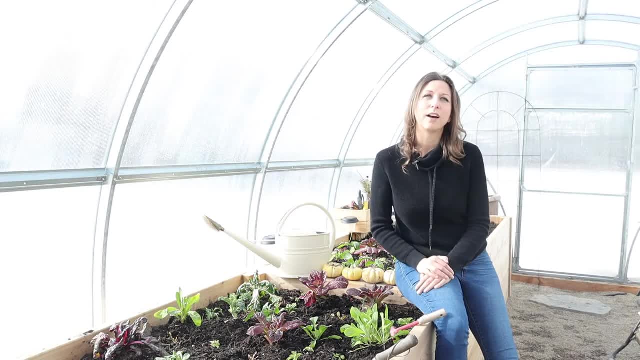 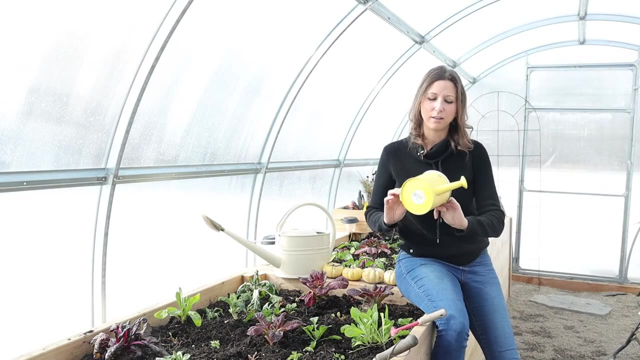 actually trying to do a good job. So maybe not at the beginning, but if you find that they like what they're doing, you might want to get some practical, like functional, kid friendly tools to use that are little versions of yours. My younger daughter- actually both my daughters- love this. I have to. 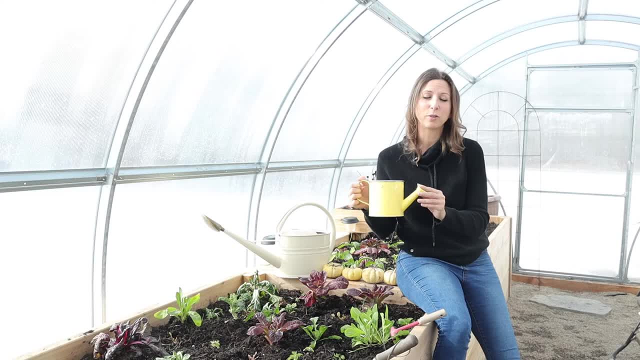 get another one now, because my, my two-year-old, almost three can now water as well, so they fight over this watering can all the time. the other, our other watering can, which was plastic, broke. of course I don't- I typically don't buy anything plastic in the garden for that reason, So I need. 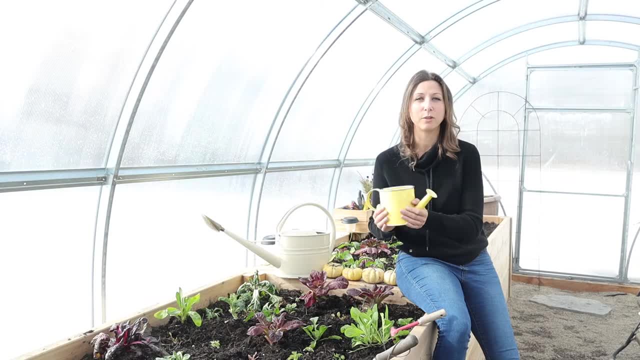 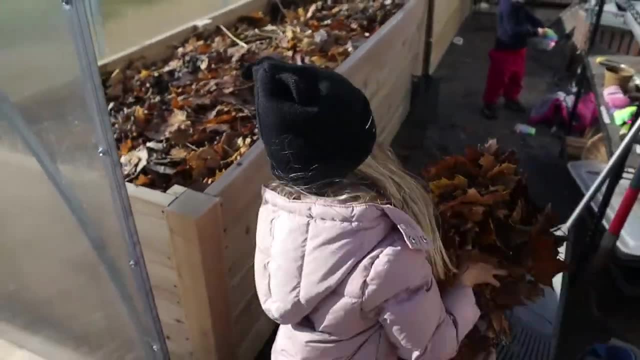 another one like this that will actually last and that will actually allow them to both water together and not constantly fight over the watering can. So, yeah, I mean anything that I do, like if I'm building a new raised bed, if I'm when I was building this greenhouse. if you've, I have a video where I showed how I built this greenhouse and 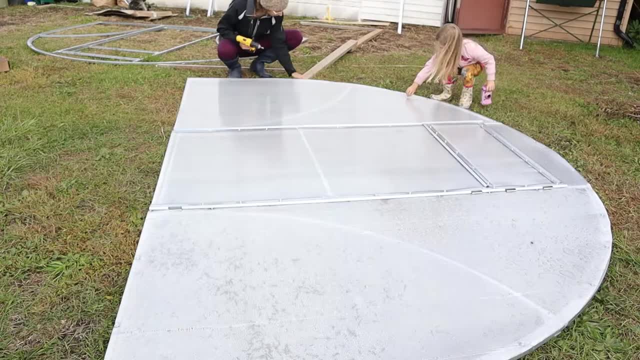 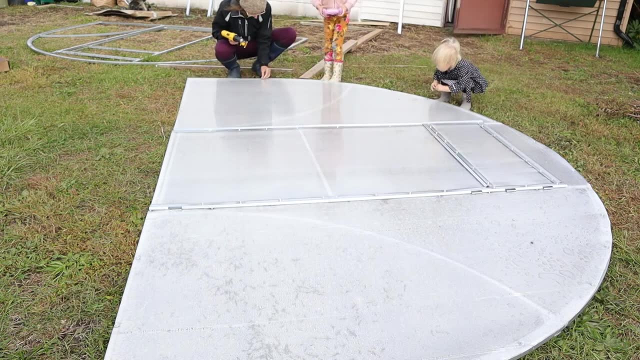 you'll see my kids kind of running around through the shots like they want to be involved. So anything that I do in my garden that they can help, even in the smallest way, I will definitely encourage and welcome their help. And then when it comes to like harvesting and actually eating, 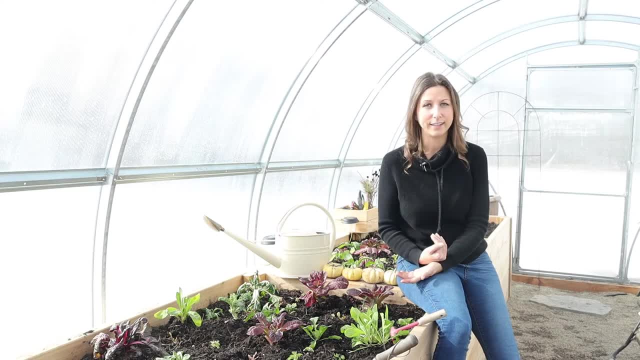 the food from your garden. you might instantly think, like I did, But I right away thought: okay, my kids are going to want to eat strawberries and they're going to want to eat, like, really sweet varieties of plants, things that they typically want to eat from the 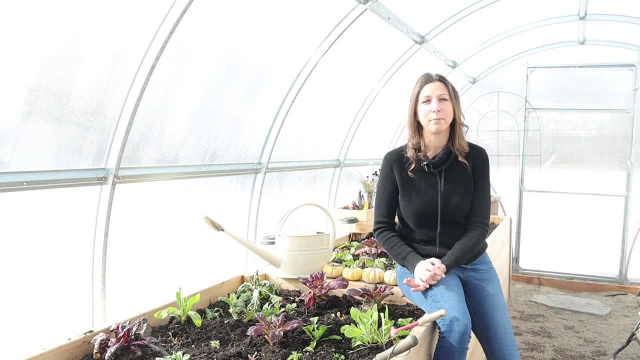 grocery store And I was surprised when I had my own garden- and I had because I grow a lot of very unique varieties of plants. I think it's very cool and also I grow year-round, so typically I'm growing things that aren't as commonly available in supermarkets. But I found that when I started 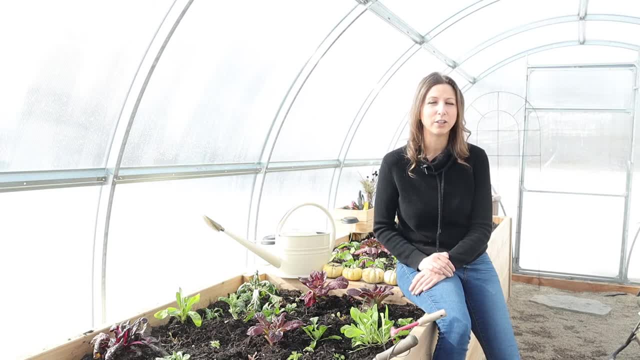 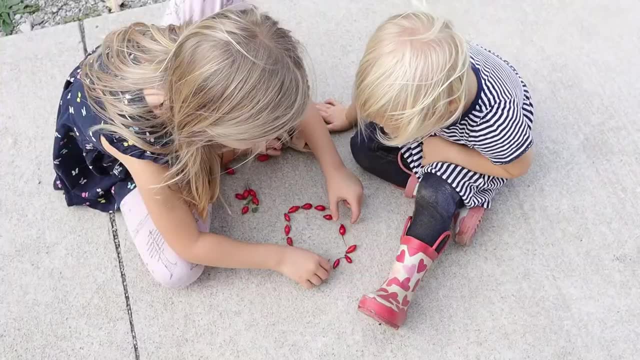 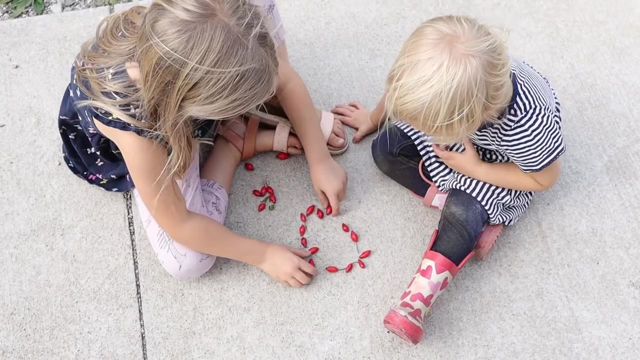 growing my own food. my kids ate a lot of very unusual things, Things that I would not have presented to a two or a five-year-old or a four-year-old or a three-year-old, any, any little age, any young age, And I was really surprised to see that they were. they loved. 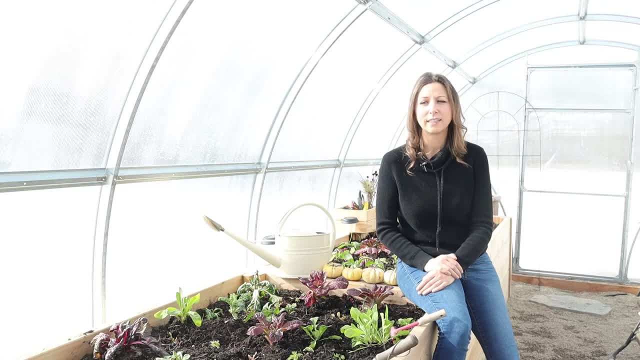 some of these unique varieties in my garden. So one of them is sorrel, and I talked about this in one of my other videos. But my kids devour sorrel from the garden and I've never had sorrel from the grocery store. It doesn't last very well, like it doesn't ship well, so it's not. 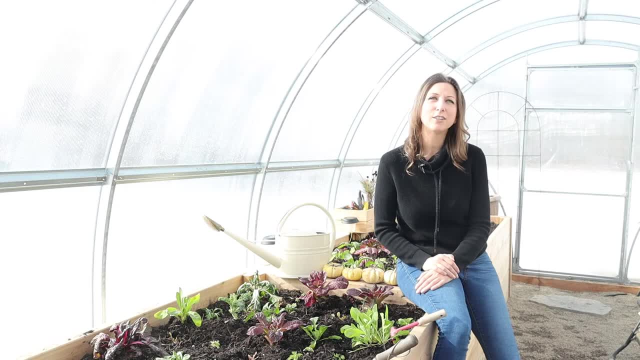 it's not. it's also not a super popular vegetable, But it has a really lemony taste, like it's got a really like a zing to it and it's not bitter. it's not spicy like. I love arugula but it's too spicy. 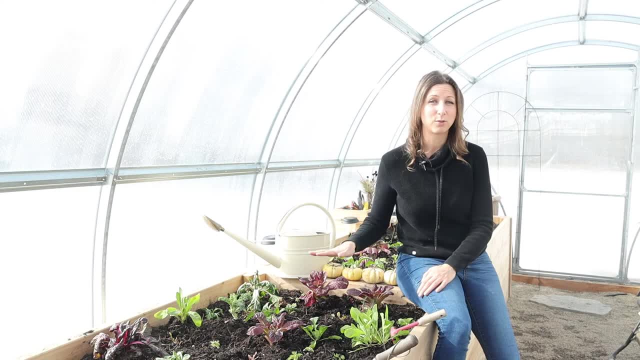 for my kids. So they just destroy this sorrel plant, like I can't keep enough sorrel in my garden right now to possibly, um, to possibly, um, sustain the two of them, And it's one of the few that my two-year-old will eat, So I'm going to show you how to eat it. So I'm going to show you. 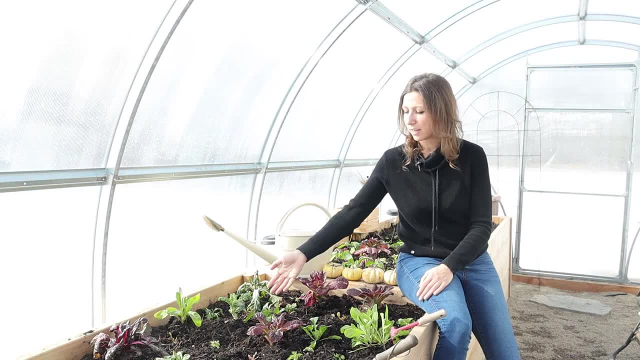 how to eat my, my five-year-old's, more adventurous. Another one is kale. Like my kids will eat they like I can't keep enough kale, at least right now. Last summer- I think it was last summer- my older daughter saw kale and she's like: oh mommy, can I eat this? because I always say, make sure you ask. 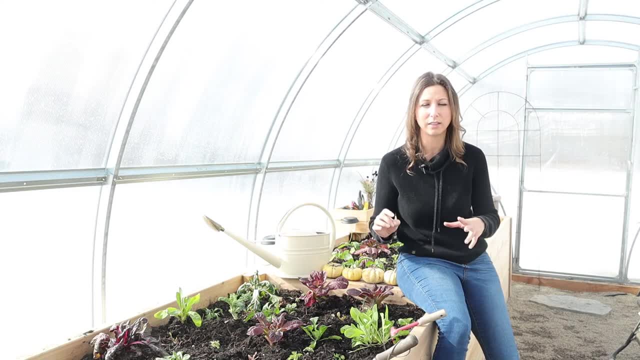 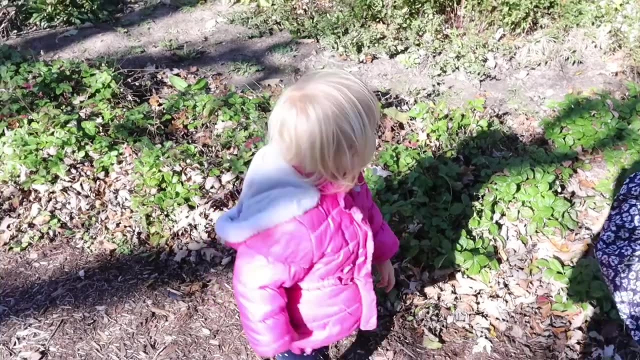 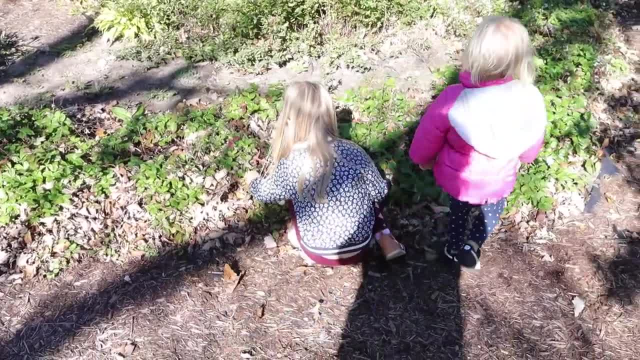 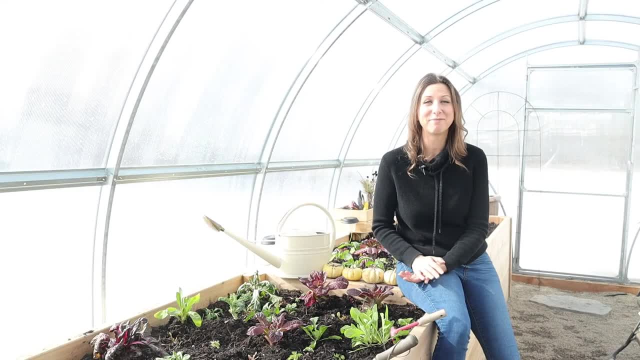 this edible, or you can only eat this. eat this edible, or you can only eat this berry, or you can only. you know you or not? I think she's going to like it. I just want to like it. I just want to try. 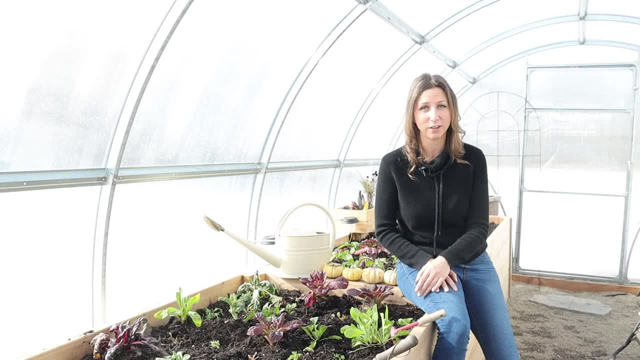 like it. I just want to to see what her thoughts are, And she loved it. She's like: Mmm, this is delicious And I have never once seen her. you grow it yourself. it's oftentimes sweeter and, if it's the right time of. 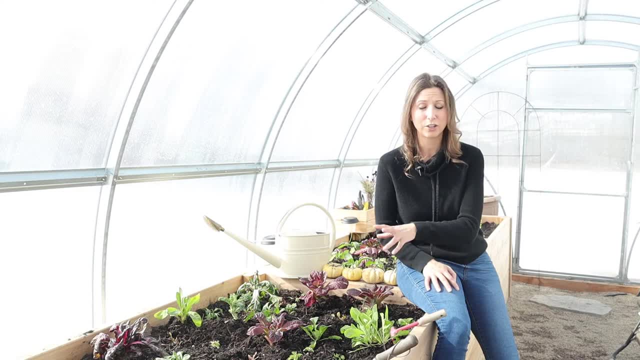 year it's got a really, really nice taste to it. I don't particularly like kale in the summer, but in the colder months of the year kale is really good right off the plant. so I was surprised, but they both now love to eat just kale off the. 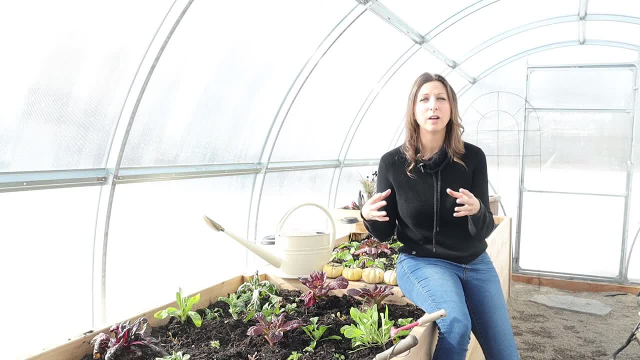 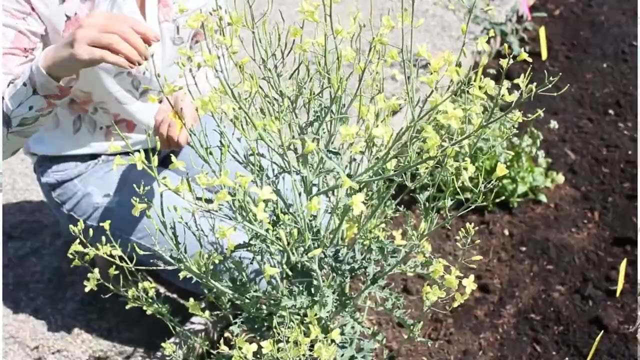 plant same thing with the flowers. so all brassicas like kale, cauliflower, broccoli like kohlrabi, they all produce flowers which have a really broccoli esque taste to them, but they love it. they were like devouring these flowers off of the plants and it's, it's funny. it's just not the kind of thing I would. 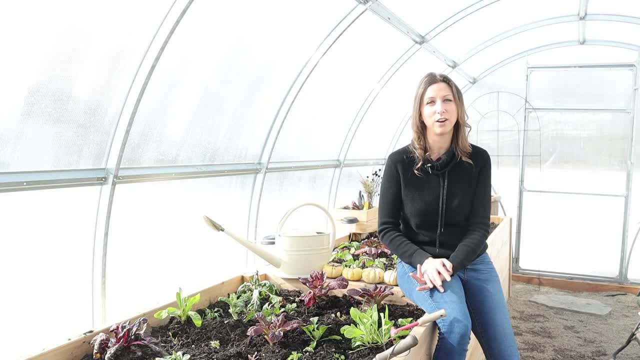 have given to my little kids to say: go and try this from the garden. so I think when it comes to harvesting, let them kind of explore and do their own thing and just see what kinds of things they like. yes, my kids absolutely eat all of our strawberries, all of our berries we have. you know, those are impossible to. 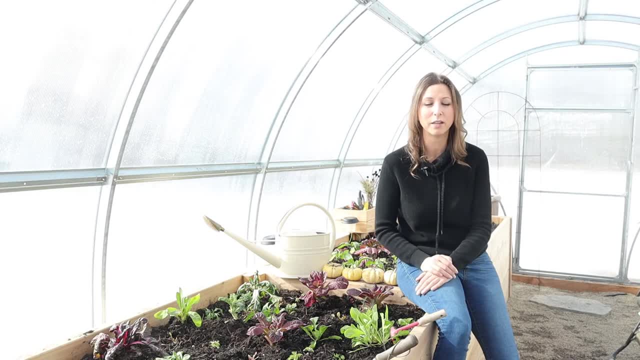 keep around if you have kids like they're like the birds, they'll snatch them before you ever see them. and also like peas. peas are another really good one for little kids. baby tomatoes like cherry tomatoes, another one for really good for your little kids. but don't. 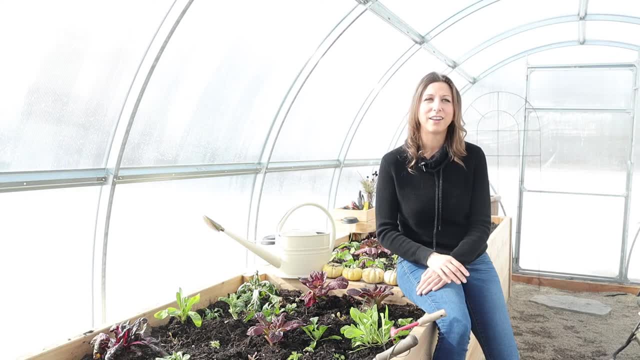 discount some of these other vegetables. so that would be my recommendation as to getting your kids eating more out of the garden. just just try it. and even, you know, go through a seed catalog with them and have them pick plants with you, especially if it has pictures. say, would you know, pick something that you want to? grow this year and then just pick what you want to grow this year and just like pick your garden. so let me on that, I'll do that for you guys. so next up, we have some really cool things about vegetable gardening I'm going to show you guys. 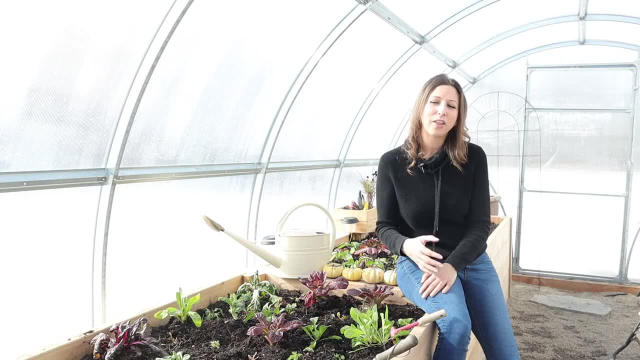 three things about vegetable gardening I'm going to show you guys. so let me, on that, obviously make sure it's a plant that would work well in your area. but you know, let them choose right, or even give them a few choices, say like, do you want to grow this, this or this? and then let them choose and actually be part of that. 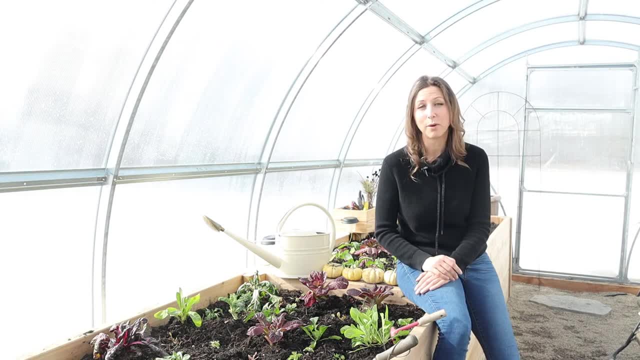 and then I can you know they'll probably be much more interested in eating it if they took part in picking it, if they took part in planting the siege, which I love. my, you know, my kids love to do with me too, if you're gonna have your kids. 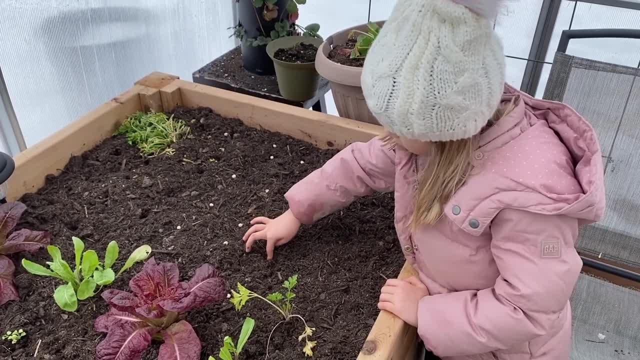 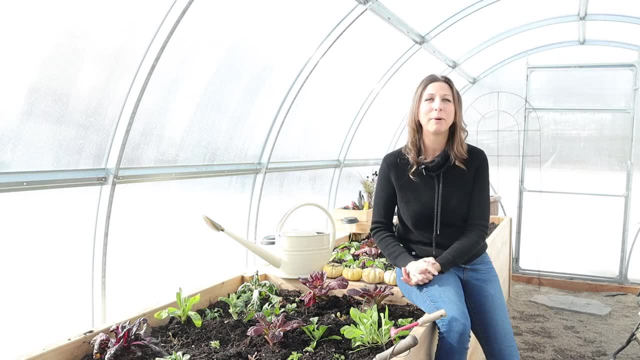 help you with planting, then I would plant a little bit of extras, because oftentimes they'll just dump a whole ton of seeds in one little tiny seed cell, which isn't ideal. but so just make sure you grow a couple extras, and if the ones that they grew didn't turn out, then that's okay. no big deal, but just having. 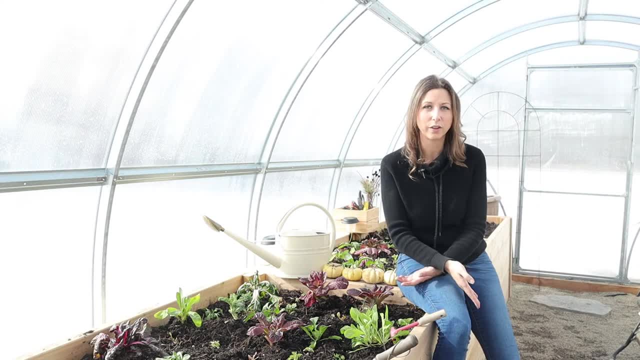 their involvement. they're not going to remember that that's the one that they planted and this is the one that you planted. they'll just remember that they took part in it and seeing the progression of the plant growing, you know. and then I think, just making sure that we're letting the kids be kids. 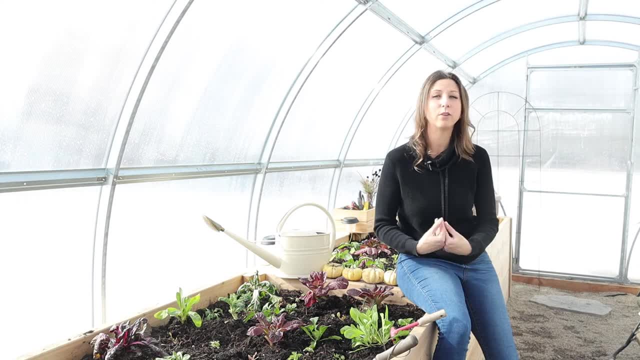 right not making gardening a chore, like I don't feel like I'm doing a good job of doing a good job of doing a good job of doing a like gardening is a chore for me. I'm doing it because I love it. I love my garden, I love spending time with my plants in my greenhouse. I love spending. 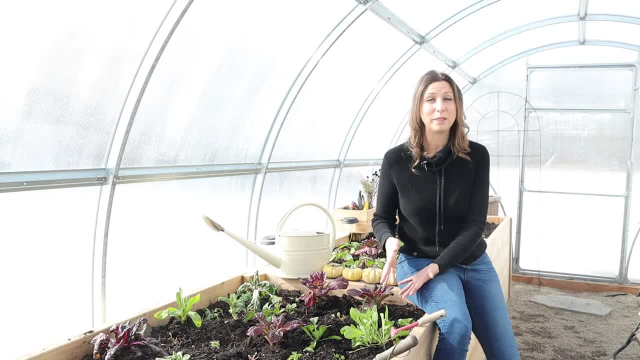 plants time with my plants outside in my garden. I just love being out in my garden, with the exception of, you know, maybe some like terrible pests or like some you know, catastrophic problem with my garden that I, you know, unforeseen issue, I don't see many of the chores or some of the many of the tasks that are. 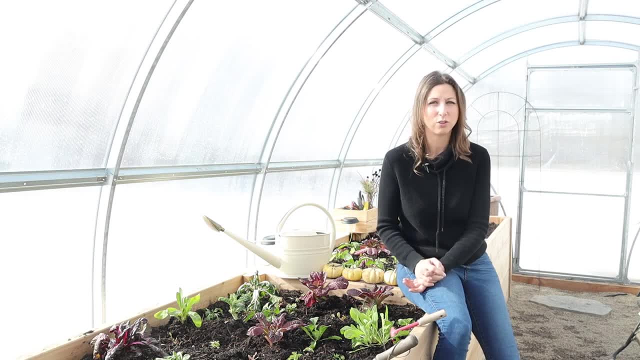 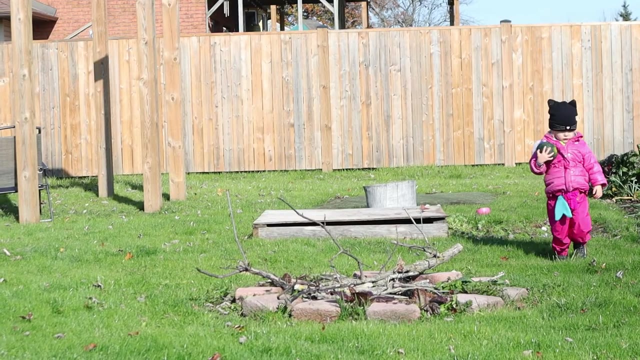 involved in gardening as being painful or or not enjoyable, because I try to make the best out of everything and if I don't like something, I try to find a way that to do it, that I do like it and I have actually grown even more my love of plants and my love of gardening because I tried. 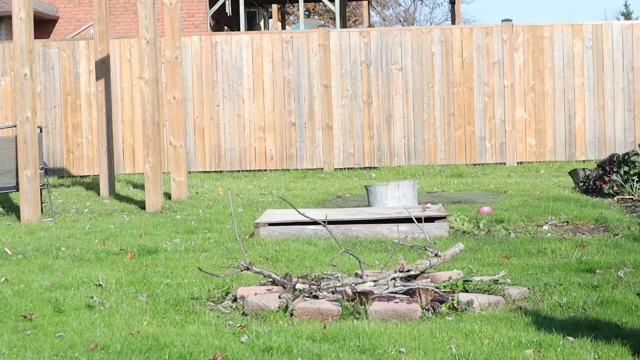 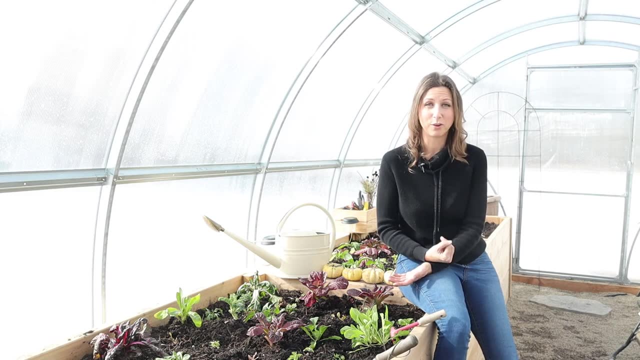 very much tailor it to my own personality, so I want my kids to also have that same love of gardening. it's funny: my husband and my husband and I- are both golfers- my husband's in the golf industry- and we're also trying to get them into golf right now and we're doing the same thing. 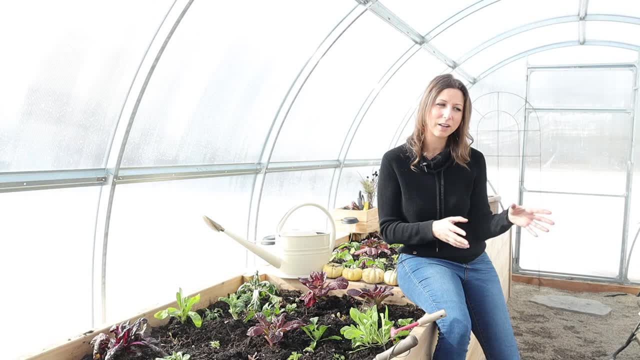 thing we're like: how can we teach them how to golf but not make them hate it? you know like if your parent is like forcing you to practice all the time or forcing you to like play and you don't feel like playing or something like that, that is the last thing I want. so same thing with my garden. 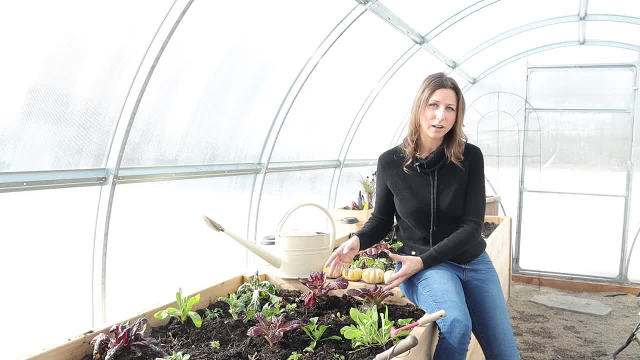 I want to find, I want to make it so that they enjoy their time. it's something that we get to do, that's fun together, because, you know, little kids like to spend time with their parents especially. I don't. I don't know, I'm not looking forward to the day when they're like mom. I don't.